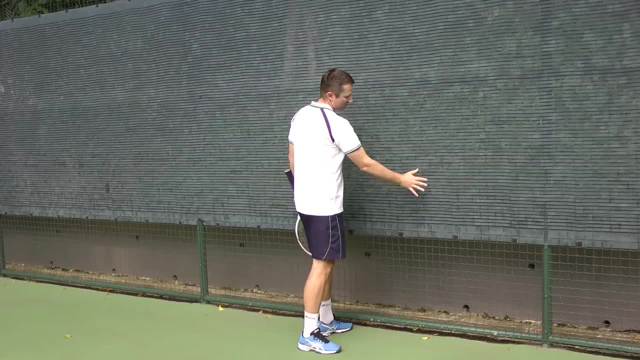 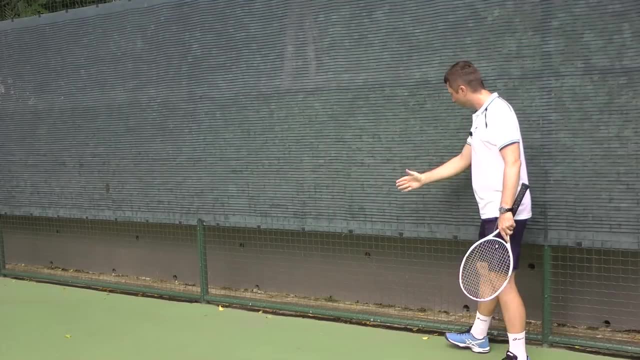 it mean ideal strike zone. So ideal strike zone, and why do we have the most power? That is just the way our body is built. so you can just try how you can generate power. You can try the same on your backhand side. So here I press in the wall. I feel this strong. then I go here. I feel not very strong. 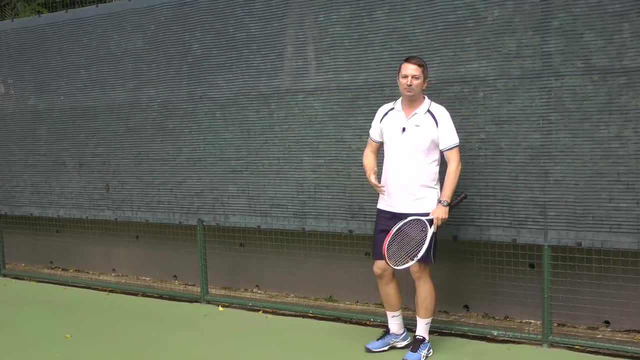 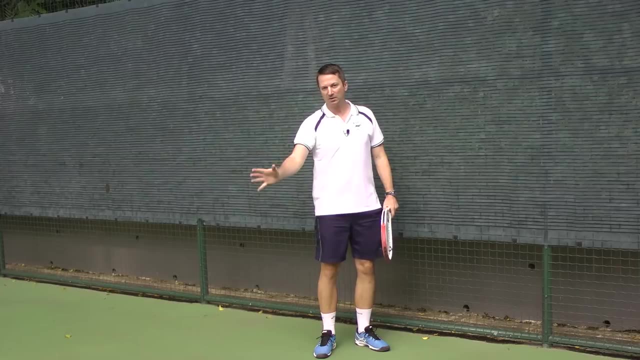 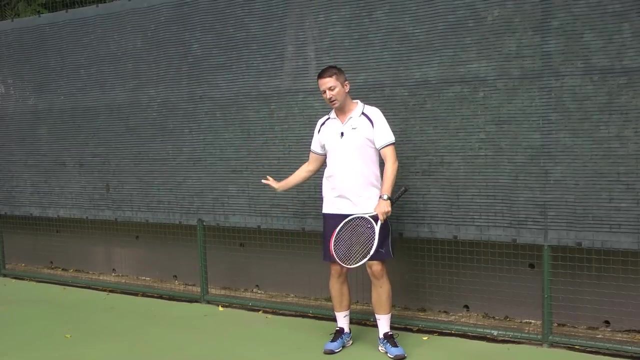 Or if I go away and I lean, I don't feel very strong. So that's how our body is built, and we will feel the most power in our ideal strike zone, so somewhere here. We usually say between the knees and the shoulders, so somewhere here, but you can be even more precise. 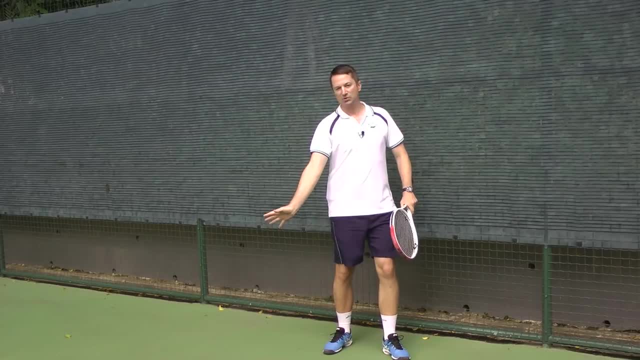 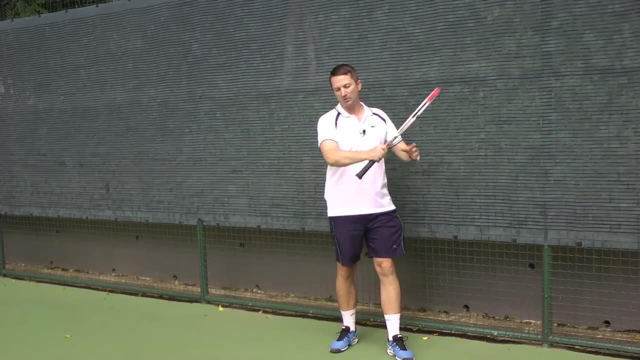 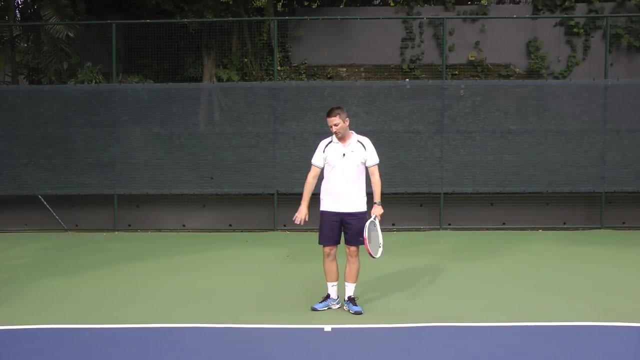 and say it's around my hip height. so somewhere here is the position for the body where we can create the most leverage and therefore the most power. another way we can find our ideal strike zone is is when we just swing the arm. so you all just demonstrate a little bit. I'll just swing my arm in the most. 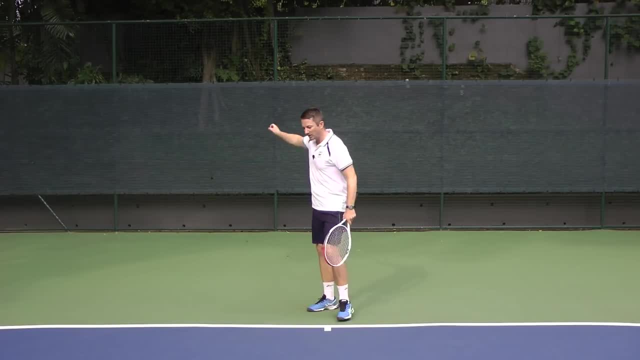 comfortable way, as if I was throwing something with an underhand throw or like feeling like I'm bowling. so if I just swing my arm in the most comfortable way and then I see at what height that happens, that will be my ideal strike zone. so I don't have to alter my swing, I just go with gravity. 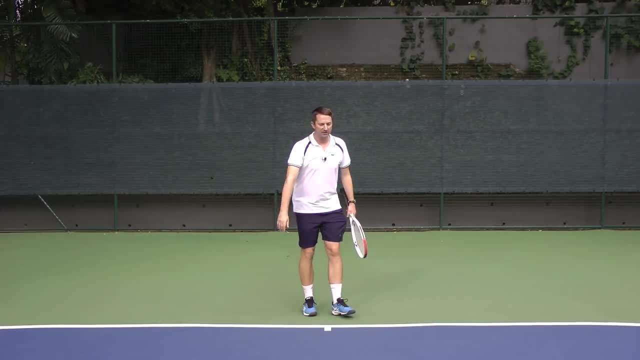 and I just swing my arm. this is my forehand side. I can do on the backhand side, so I just I just swing my arm in the most comfortable way and then I see my body and then I find my balance. we go from right to left and we go from. 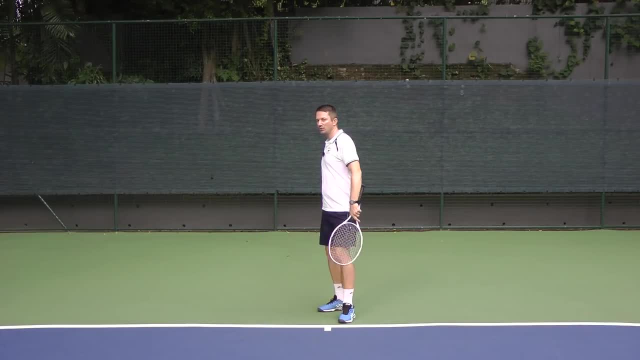 oh, this is the height. so if i want to change my swing and i say, okay, i need to, i hit a high ball. you can try and swing your arm and you will see that it's a bit less comfortable to swing here than to swing here. and so, because this is the most comfortable, 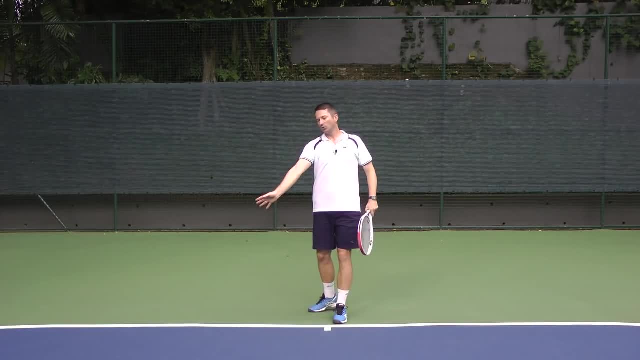 height or position to swing. that's why my stroke will have the most effortless power. so again, if i just if i just swing my arm comfortably, then okay, it's going to swing. here i can try a high back hand and you will see it's not very comfortable. so that's why we don't have power when we have a. 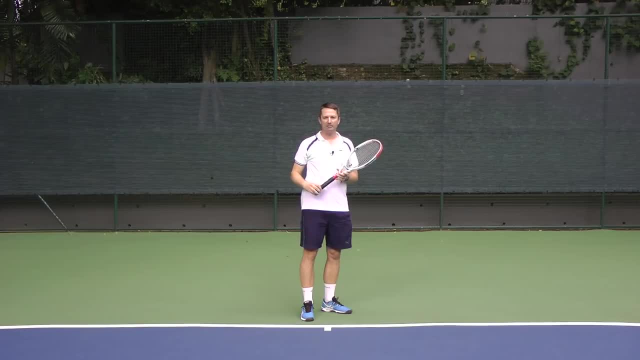 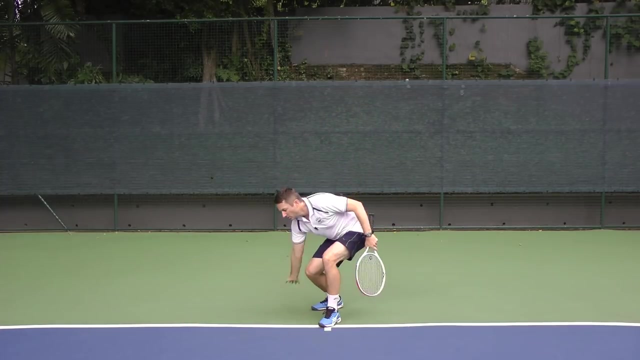 high backhand, and so don't even try to hit high backhands with power. just try to hit them back and try to position next time or wait for the next ball that comes in your ideal strike zone, and then that ball you can hit with power. so again, you can also try, like to swing very low. 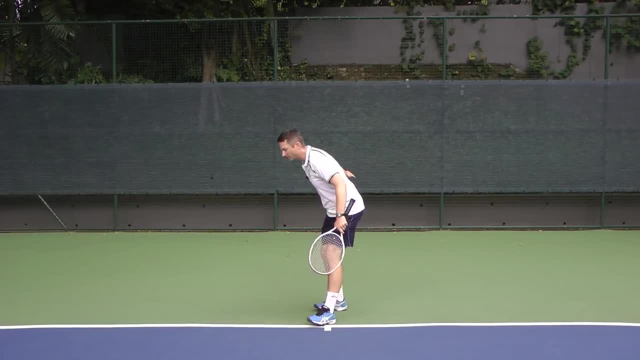 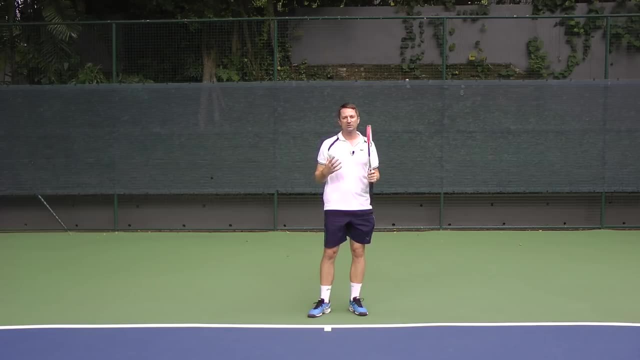 and you will. You will feel that your body is not so comfortable, and especially if you swing away. So these are just little exercises that will help you really understand. why do we want to hit the ball here? It's because our body is built the way it's built, and if we swing- which is what we want- 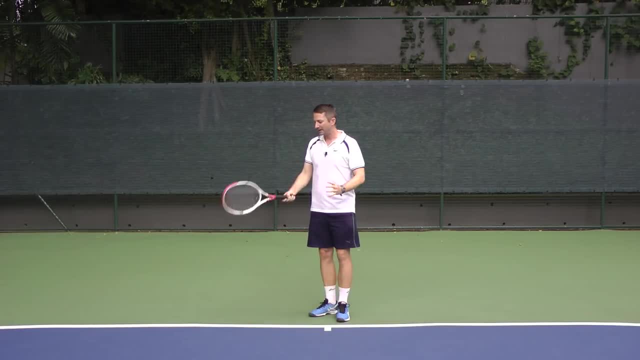 when we hit forehands or backhands, we don't want to just mechanically execute them, We want to swing our arm too. And when we naturally swing our arm then we see at what height that naturally happens. So if I get the ball at this height, then I will have the most power and the most control. 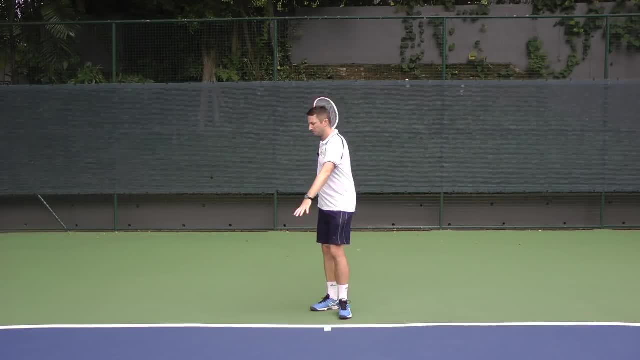 The reason why I will also have the most control is because in practice- in reality, when I play, I will hit the most balls at around this height. So this is my most grooved swing. I've hit this forehand The most times in my life. 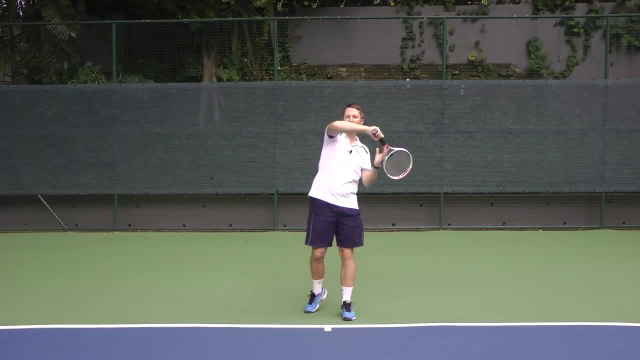 I haven't hit this forehand or this forehand as many times. Therefore, this forehand, at this height, at this distance, is the most grooved forehand. So if I get in a position where I can hit this forehand, then I have the highest chance. 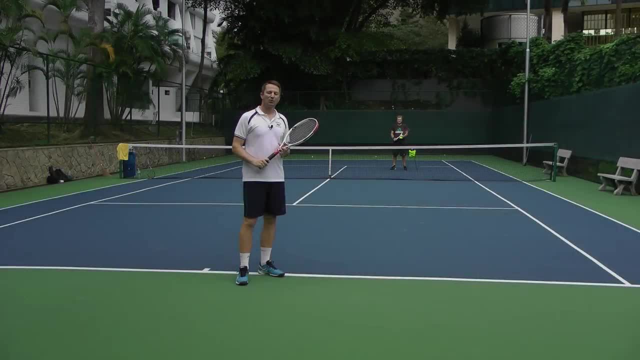 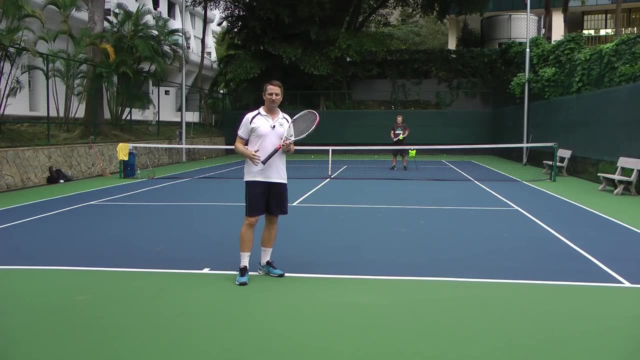 of making the ball go in. So what are some of the reasons why you might not be hitting the ball in your strike zone? The first one is that you might not be hitting the ball in your strike zone. You might not know about it. 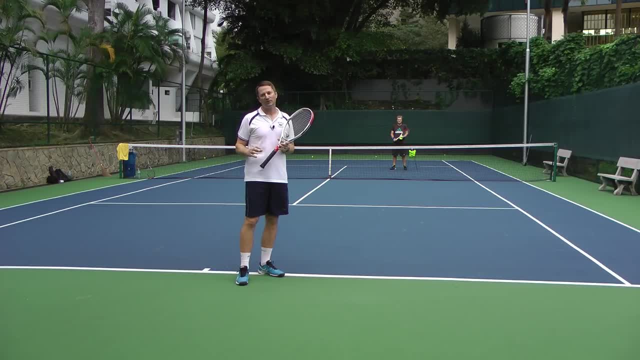 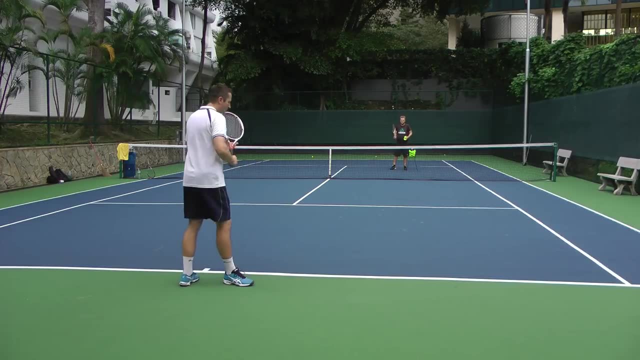 And if you don't know about it, then it means that you also don't feel the difference between hitting the ball outside of your strike zone or inside your strike zone. So when you're not hitting in your strike zone, then the ball is like this: 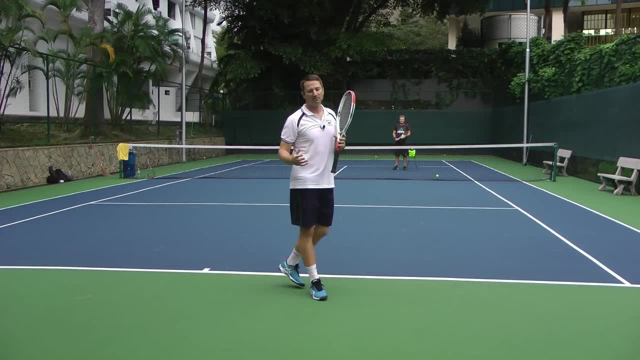 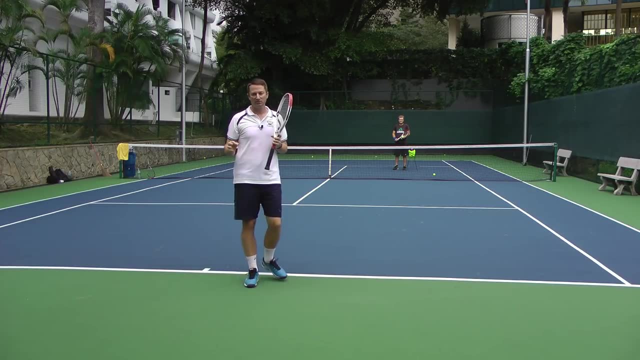 And you say: well, this is good enough, I reached the ball. So if your goal in your mind is just: the balls is coming towards me and I need to reach it right- the minimum amount of effort required to do that. So if you just think I need to reach the ball, then this is what will happen again. 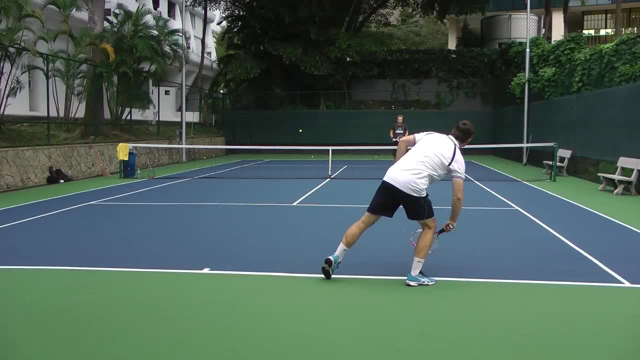 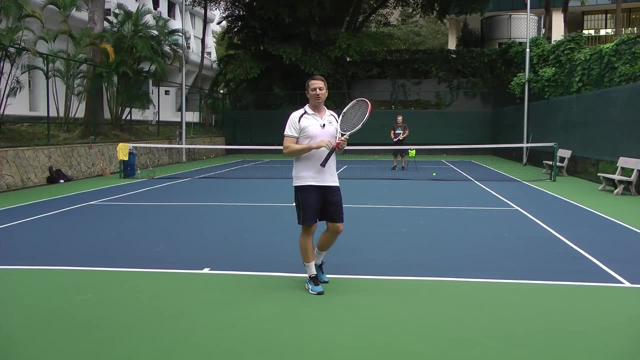 So I'm here, I'm just thinking I need to reach the ball. Okay, I got it. I reached the ball And you think, well, that's good enough, I played over and maybe something's not right with my forehand. 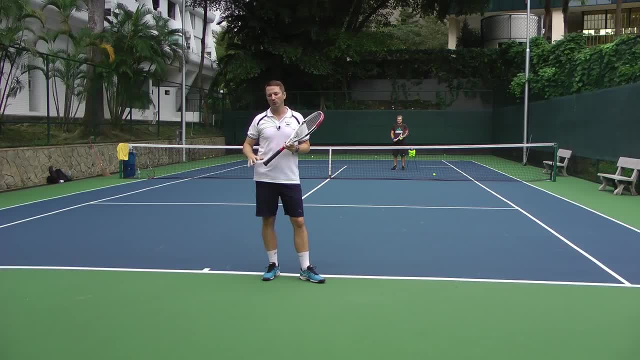 I need to work on my forehand, But that's not the case. You were off balance and you were not hitting in your strike zone. Okay, You cannot generate good, effortless power outside of your strike zone. So when the ball comes next time, if you get in a position and you hit the ball in your 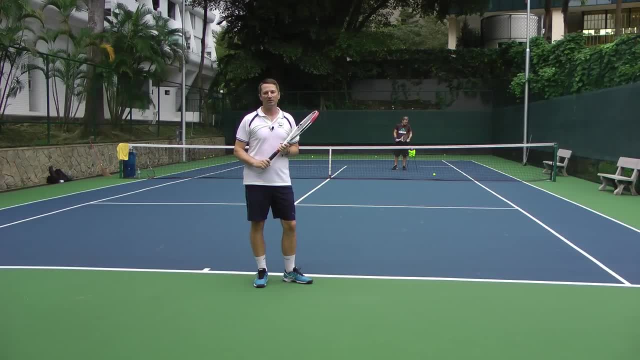 strike zone, then you will get very nice effortless power, And so the reason, for example, why I play in my strike zone as much as I can, is because I can hit a better shot. I can hit a better shot and I can hit a more effortless shot. 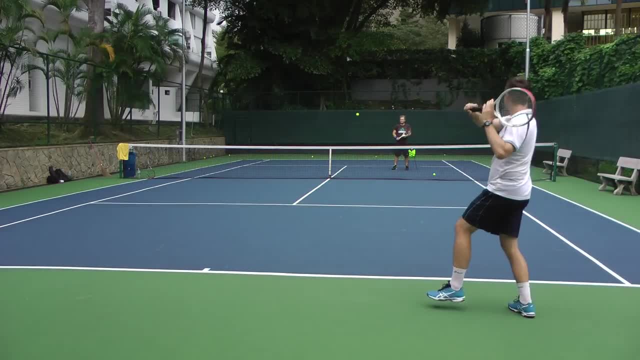 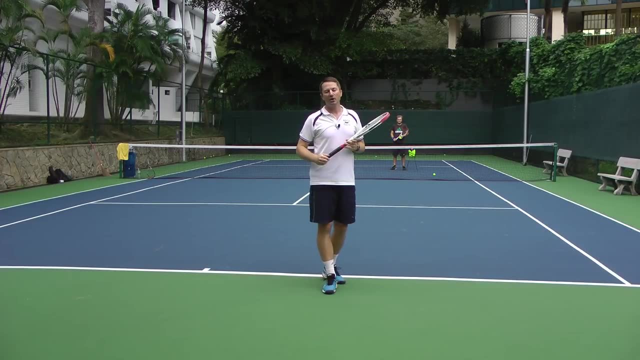 So when the ball is coming, I try to position myself In a good position, in a balanced position. I get to the ball, I hit the ball in my strike zone And I'm going to hit a good shot. The second reason why you might not be hitting the ball in your strike zone. 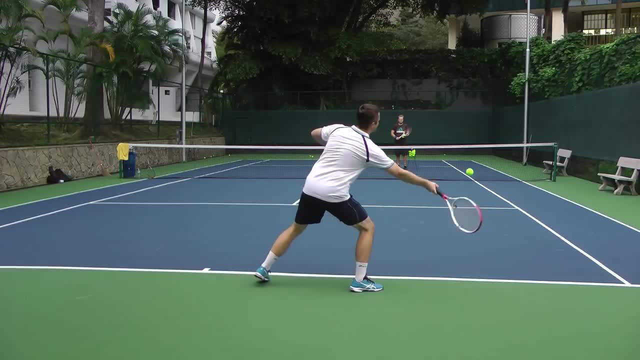 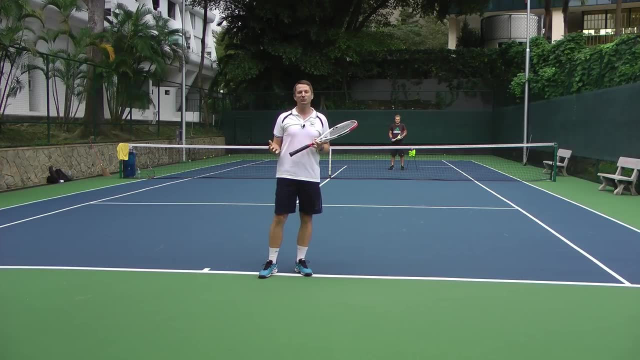 So again, it looks something like this. It looks like this is because you want to conserve energy- So I will not use the word lazy Oops, I just used it. So you want to conserve energy And you say, well, this is good. 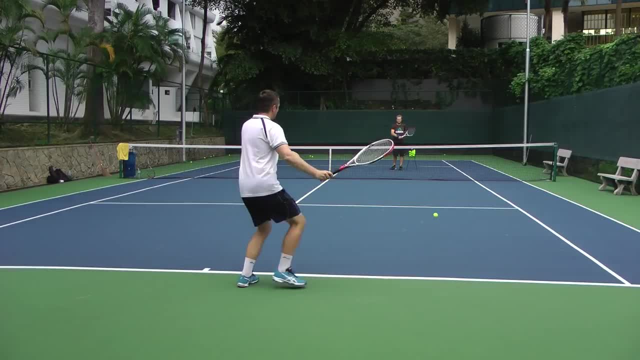 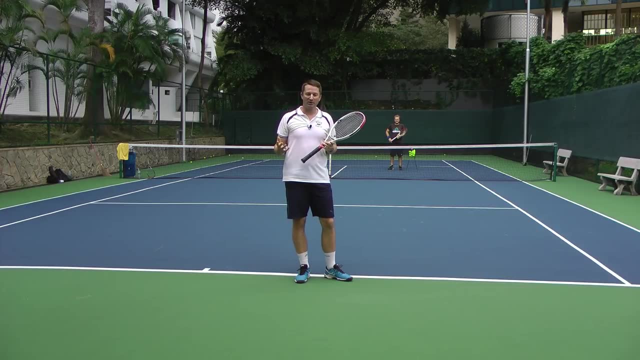 This is good enough, I can hit the ball. I don't want to suffer too much, I got it. And you want to conserve energy? Now, that's eventually your choice, but I just want to give you one message, And the message is that if you want to hit good shots, you have to pay the price for. 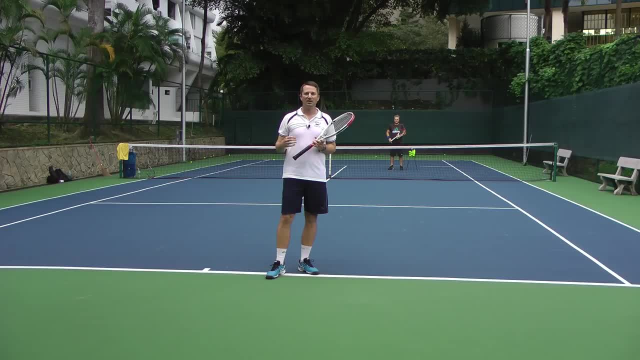 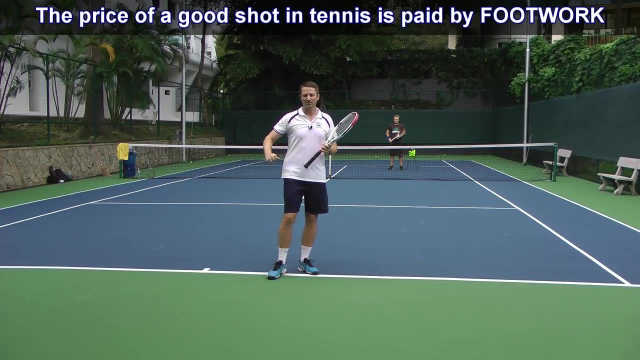 them. You cannot have good shots for nothing, And in tennis we pay the price with effort and footwork. That's how we pay the price. We don't pay the price with the arm work. We pay the price with the footwork. 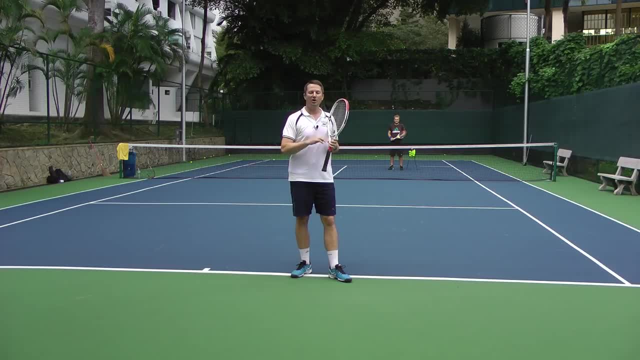 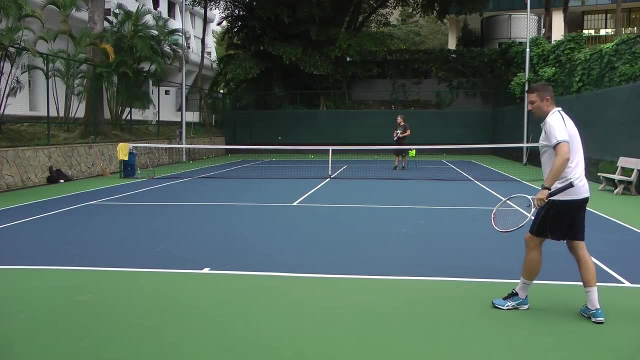 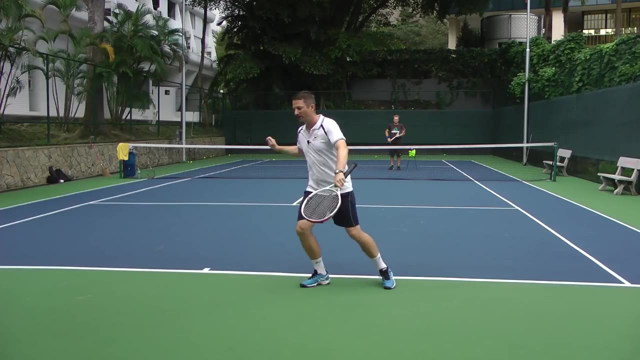 The legs work, The legs suffer so that the arm can move very comfortably. So when the ball is coming, I have to pay the price with my feet. I have to get to the ball. I need to balance myself, I need to use my muscle to stop myself from moving. 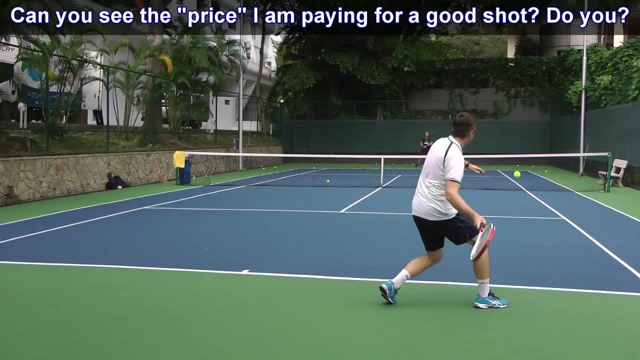 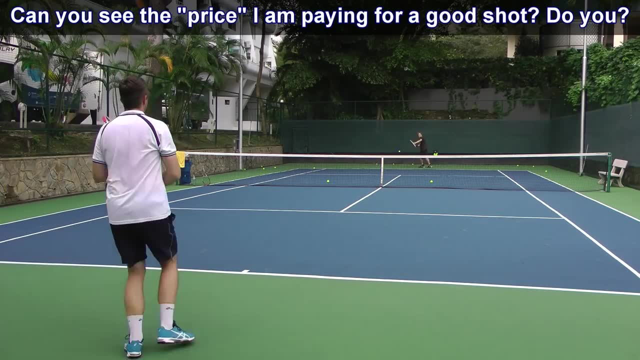 I cannot fall off the stroke, So I need to get here, I need to stop, I need to position, I need to push off, And this is the price I have to pay for a good shot. And if I hit a good shot first, I will prevent attacks from my opponent. 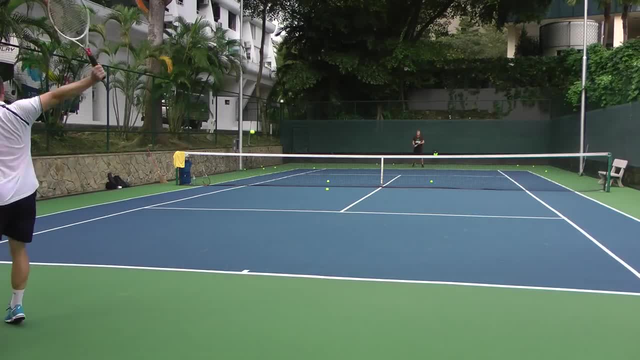 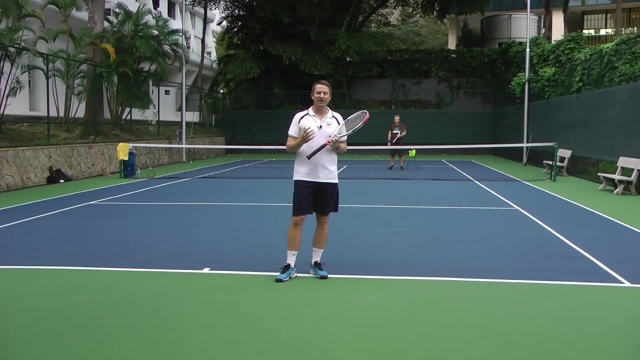 And secondly, I might force mistakes or hit some winners. So this is the message I want to send you: that you understand what is the price for playing good tennis. You have to get to the ball so that you hit it in your strike zone. only then you can. 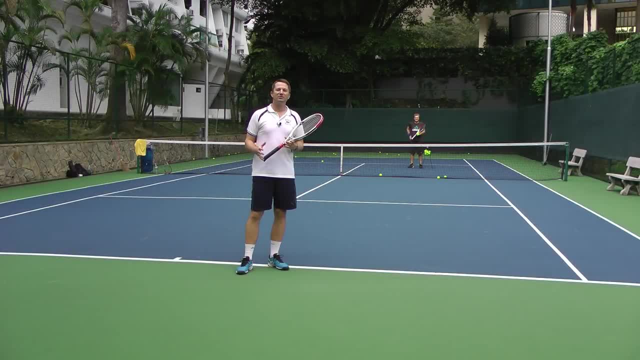 play good tennis. It is important that you know that you must have the ability to improvise too. So we try to get in the ideal position and hit the ball in our ideal strike zone when we can. But sometimes we really cannot. Even if we are not lazy, even if we try everything we can, sometimes we cannot get to the ball. 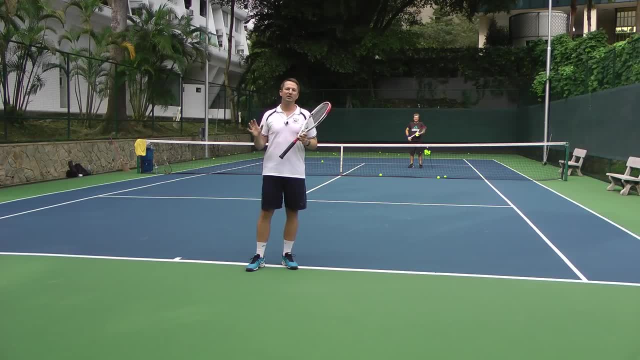 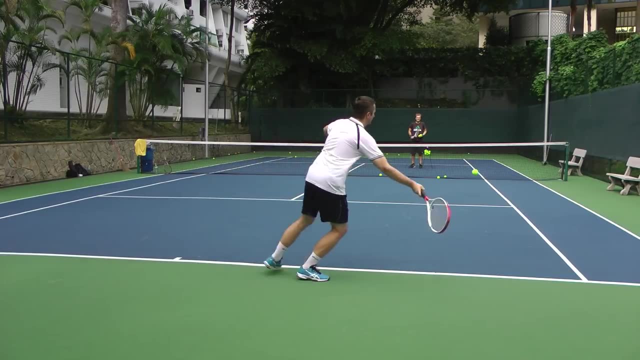 So we must be able to improvise our strokes and hit the ball with some control, even outside of our strike zone. So if I get the ball away from me And I really can't get it, Then I must be able to somehow control that ball. 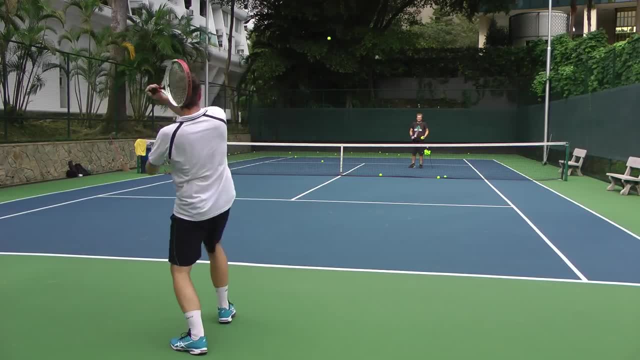 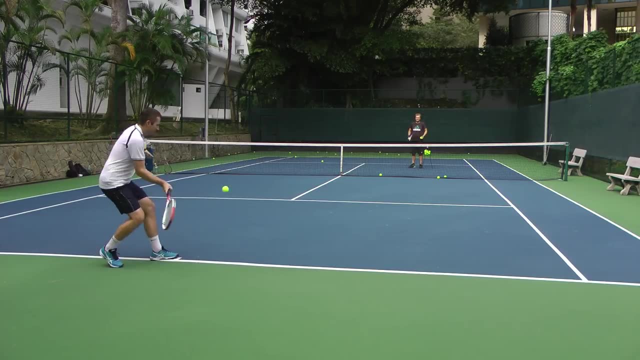 Or if the ball is like really high and I get out of my strike zone, I still must have enough feel and control to get it in the court. Or maybe the ball will come fast to me and I can't get in a position. I still need to find a way to put it over and direct it somewhere. 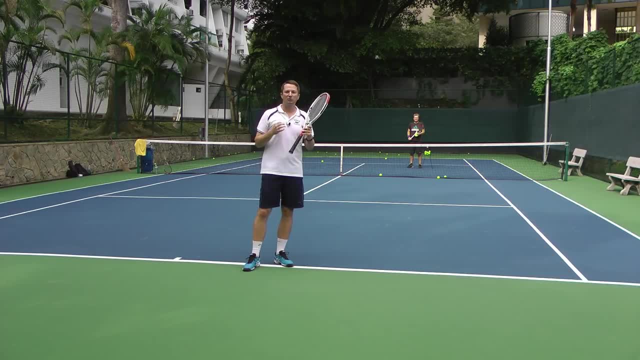 So just giving you this message that you don't feel terribly bad If you don't hit the ball in your strike zone. you must be able to improvise, But again, my message today is that you should try and get in the right position. 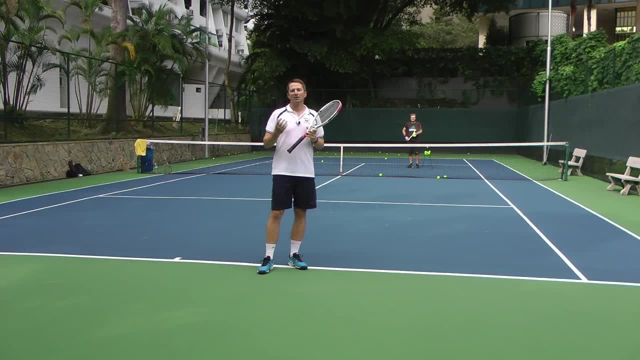 So, again, if you don't pay attention to it and in your mind, the only task you give yourself is: I need to reach the ball, then you will reach the ball like this and like this, like this, because our arm can move all over the place and reach the ball. 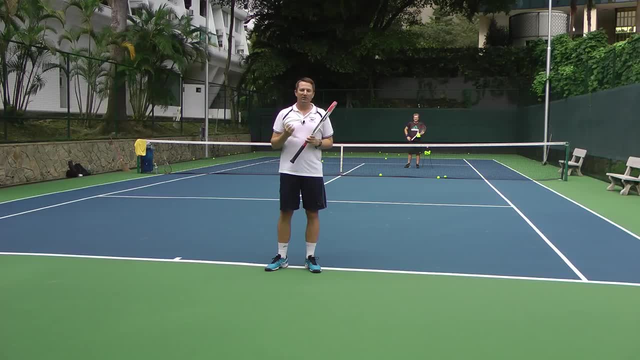 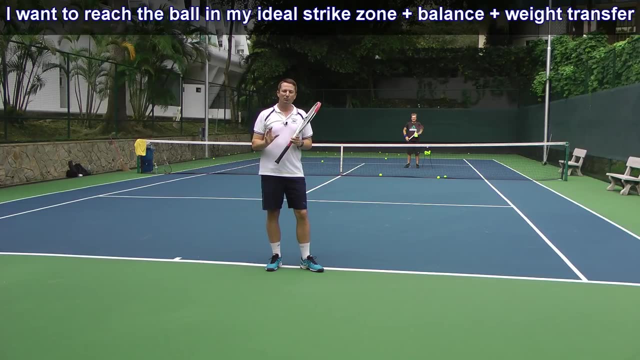 But what you need to look for is you have another. you need to have another question in your mind, and the question must be: I want to reach the ball in my ideal strike zone, I want to be well balanced and I want to feel good weight transfer into the ball. 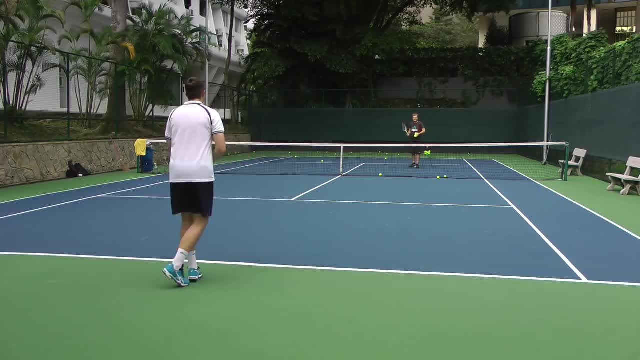 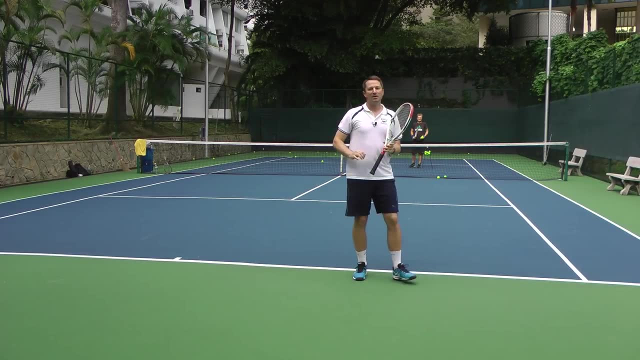 that's what I'm looking for. so when I'm receiving a ball, I want to get in a position where I feel good balance. the ball is somewhere in my strike zone. that's what I'm looking for. I'm not looking just to reach the ball, I'm looking to get to the ball. 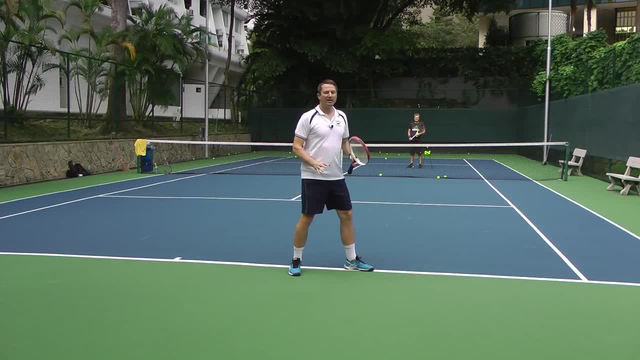 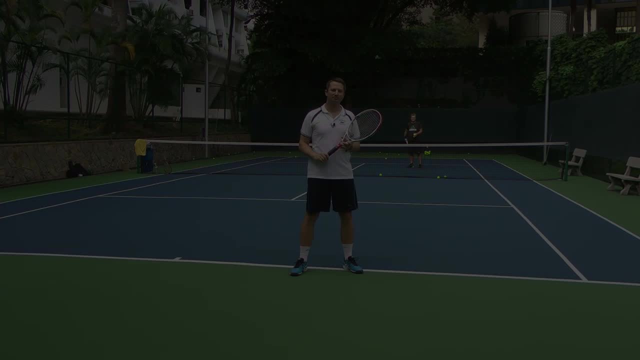 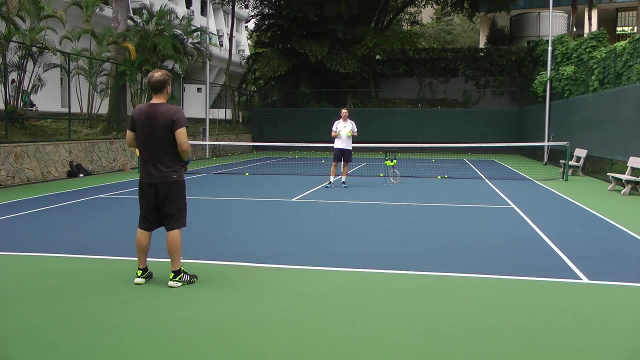 and feel very stable, very balanced and hit the ball at the right height and at the right distance, and when that happens I will hit a good shot very effortlessly. so the main problem in hitting the ball in your strike zone or not is that you learn to adjust with your arm because you can reach. 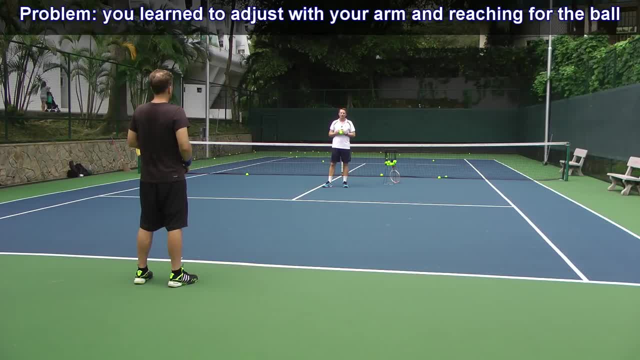 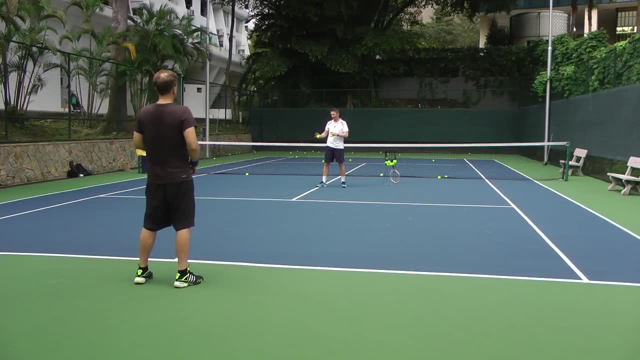 all over the place with your arm and you conserve energy. you can hit the ball here, or you can hit the ball here or here, so you are adjusting with your arm, and when you do that, you're not hitting the ball in your strike zone. so you need to learn to adjust with your feet. 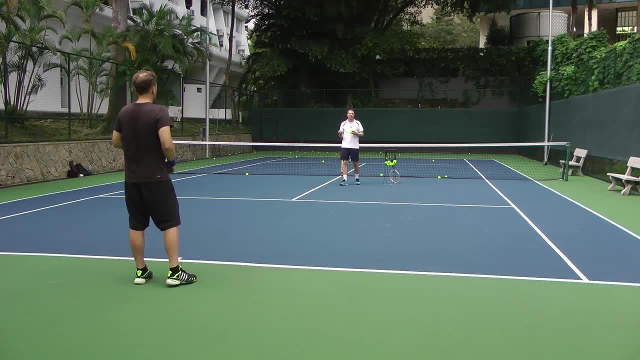 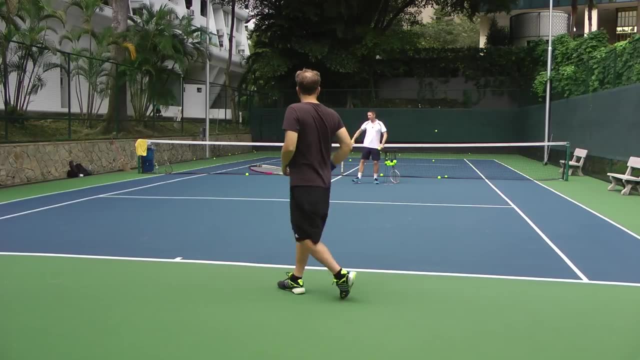 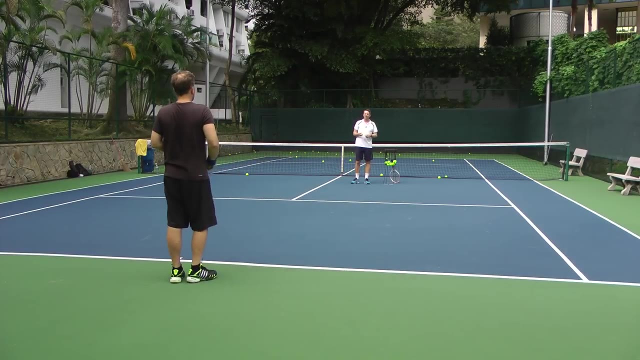 but first I'm gonna ask David to demonstrate again. what does it look like when you try to adjust only with your arm? so if the ball is away like this? so David reached the ball, but you can see him stretching and leaning, so he's not really hitting in his ideal strike zone. the ball is. 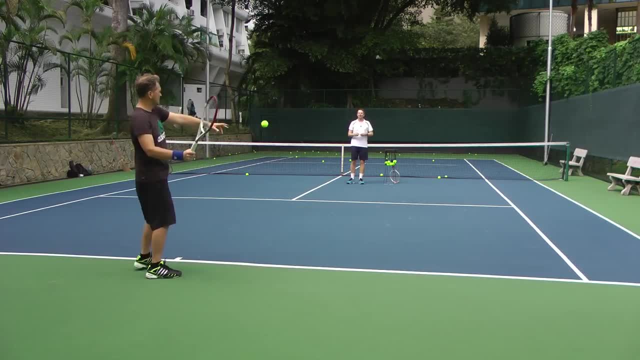 too far. or if I give him, like, a high ball, he's hitting the ball too close to him, above his shoulders. so again, he's not hitting the ball in his strike zone. so, assuming that there's a player, and they don't understand, they're so used to.